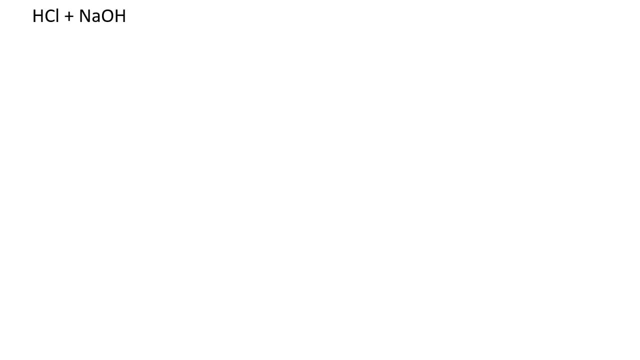 literally the way to do it. So let's start. Let's say we take HCl and NaOH. Now that is an acid and a metal hydroxide, so we know that that always gives us a salt and water. What I want you to now do is you take the salt. So you take the salt, which is NaCl. 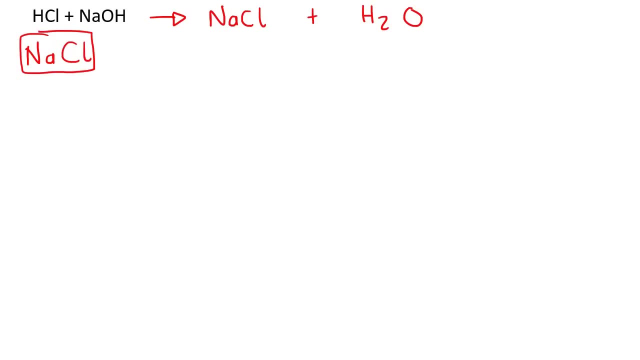 and I want you to break the salt up into its ions. So that would be Na plus and that would be Cl minus. Now what you do is you examine the Na plus. you try to ask yourself: where did that come from? Did it come from H-C-O or did it come from? 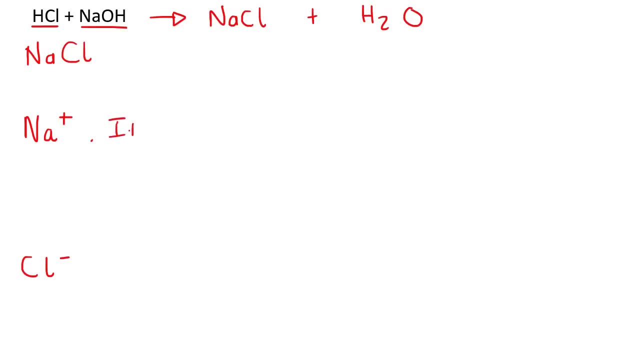 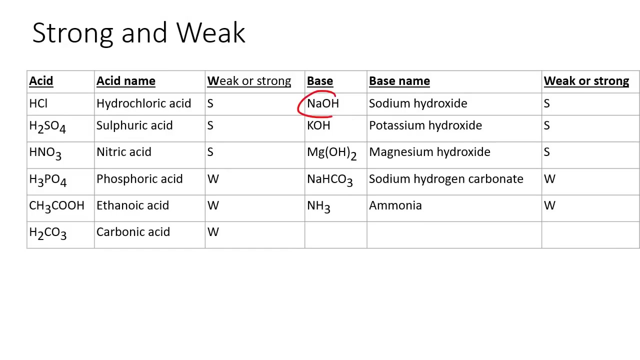 N-A-O-H. We can say that it comes from N-A-O-H. Now is N-A-O-H strong or weak? So we go back to our little table and we go to N-A-O-H and we see: oh, it is strong. So we can say here N-A-O-H. 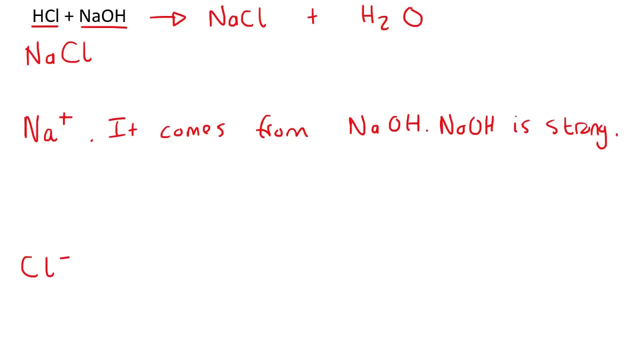 is strong. So because it is strong, we say hydrolysis will not happen. Okay, so you don't have to worry about hydrolysis. Next we go on to C-O- Now where did that come from? It comes from: 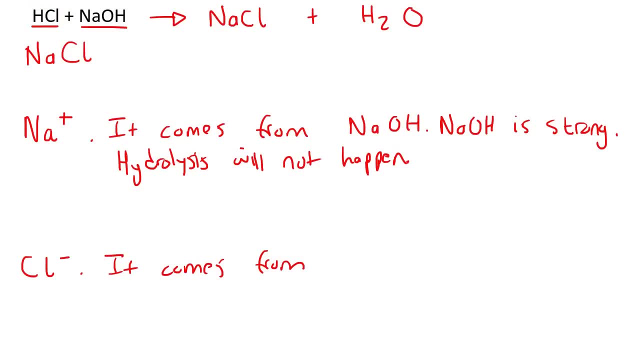 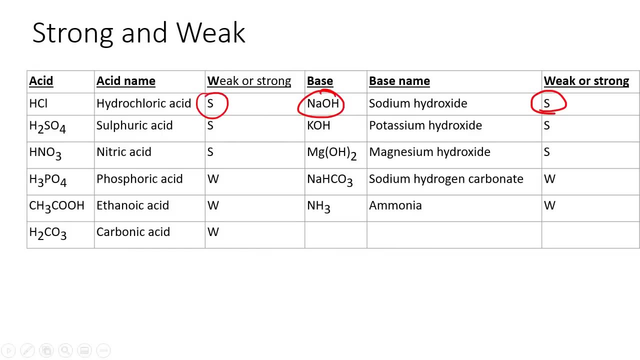 H-C-L. Okay, so it comes from H-C-L. It can only come from this one or this one. Then we go back to our table and we realize that H-C-L is strong. So we can say: H-C-L is strong. 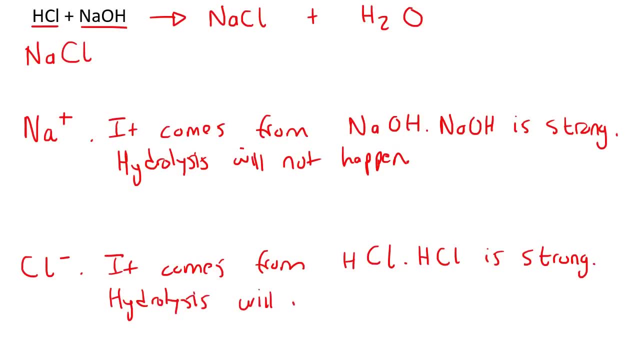 Therefore, hydrolysis will not happen. Hydrolysis only happens when something comes from a weak base or a weak acid. So if you had to do a titration with H-C-L and N-A-O-H- so let's make a little summary here. Therefore, if you do a titration, 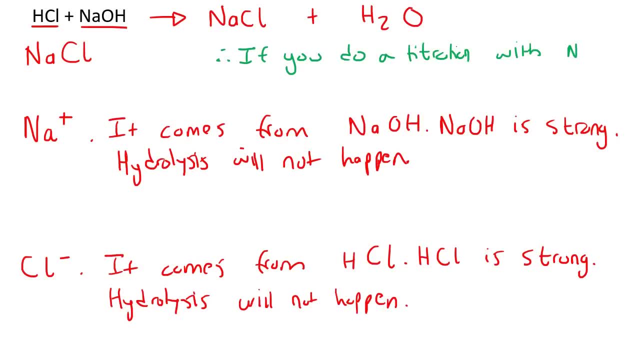 with N-A-O-H and H-C-L, no hydrolysis takes place. So therefore, the pH will be equal to seven, Or let's rather say pH at the end of the reaction- at the end of reaction- will be equal to seven. 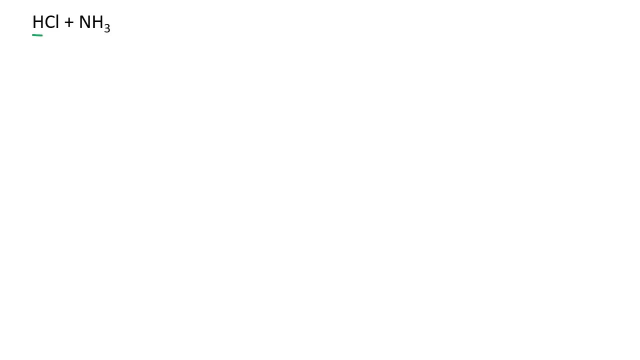 Right, so here's another example. So this is an acid plus ammonia. Now you should know from the previous lessons where we've spoken about the common types of reactions. you should know that this gives you a salt, And that salt will be N-H-4-C-L. 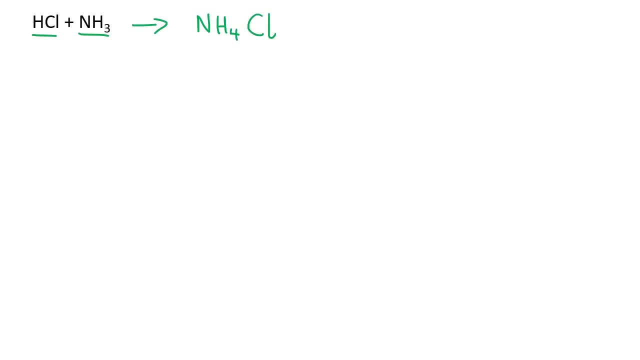 It doesn't give you water or anything like that. So what you do now is you look at the salt and you break that salt up into its ions. So let's quickly see here: So the salt is N-H-4-C-L. Now break it up into its ions, N-H-4 plus and C-L negative. Then you look at the N-H-4 and you ask: 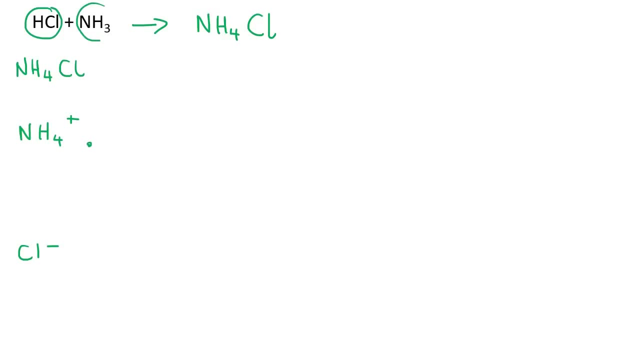 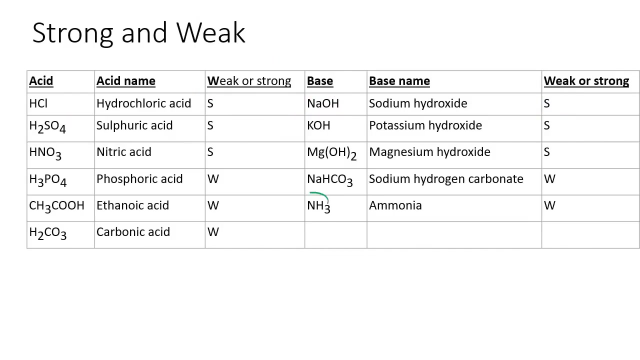 yourself: where did that come from? Did it come from H-C-L or did it come from N-H-3? It came from N-H-3.. So we can say it comes from N-H-3.. Then, if we look at our table, we can see that N-H-3 is weak. So we can say that N-H-3. 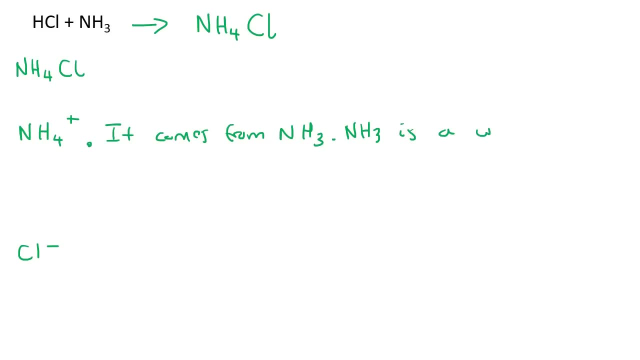 is a weak base. Therefore, hydrolysis will happen, And I'm going to show you what that actually looks like now. Hydrolysis will happen. Awesome stuff, guys. You excited to see what hydrolysis actually is? I'm going to show you that now. 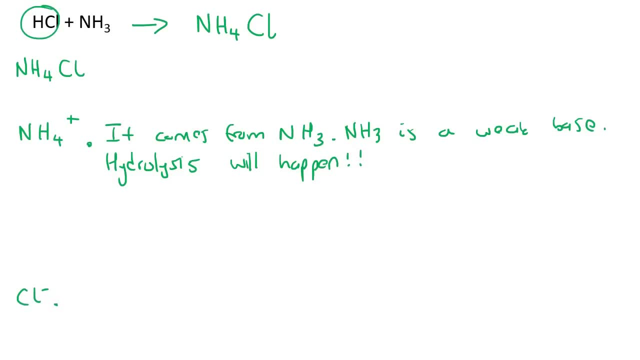 Let's quickly look at C-L- C-L- comes from H-C-L. We saw in the previous question that that is a strong acid. H-C-L is strong, And so hydrolysis will not happen over there, Alright, so what is hydrolysis actually? Can you remember that video I showed you guys, where you 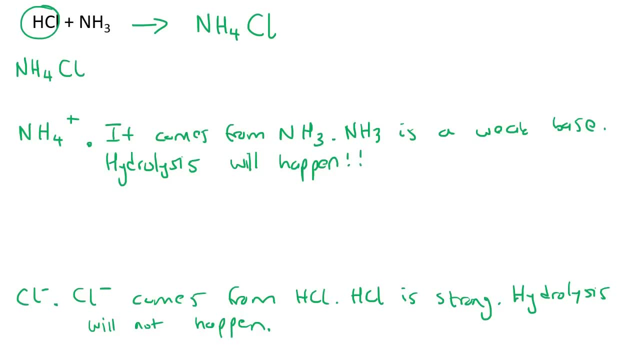 had the one boy sitting in the car and he was super unhappy to go to school. And then I showed you after that. there were those kids who were busy dancing And in that video I explained what a strong and a weak substance actually is. 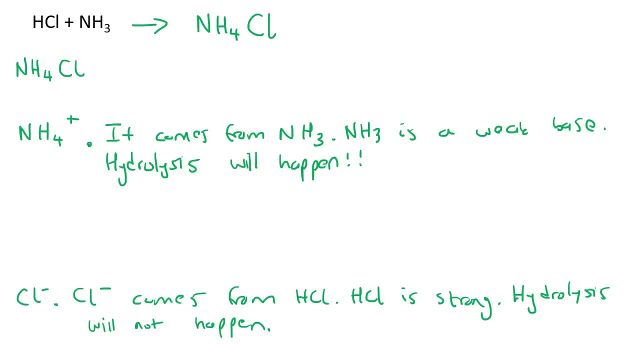 So can you remember that the weak substance is the one that does not want to react. So this NH3 is weak, So it doesn't want to react, So it doesn't actually want to go in this direction, It rather wants to behave as an NH3.. 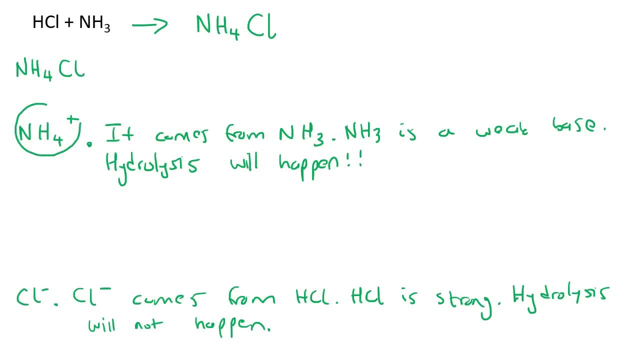 So what happens now is that this NH4 is feeling a little bit uncomfortable because it would rather prefer to be NH3. So it's going to try go and become NH3 again. How does it do that? It is going to react with water. 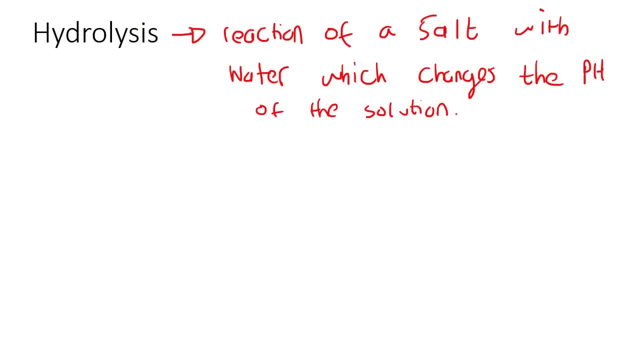 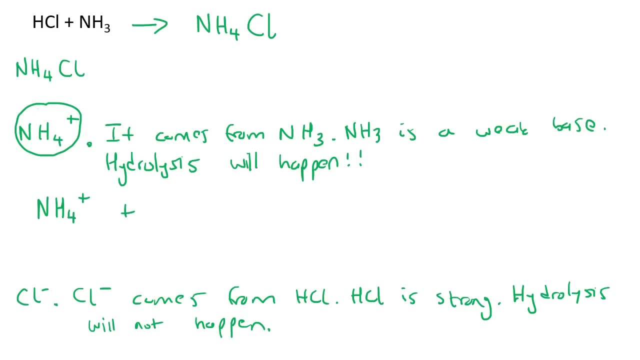 We said in the beginning of this lesson that a hydrolysis is the reaction of a salt with water. So it's very easy: You take NH4+, you react it with water. We know that the product will be NH3. And then you've got to try figure out what the other product will be. 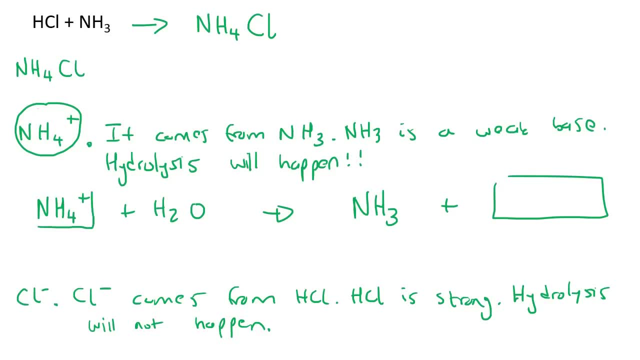 by looking at it. How did this NH4 turn into NH3?? Did it give away a hydrogen or did it accept another hydrogen? It gave a hydrogen away. That's why it now has three hydrogens. Who did it give it to? 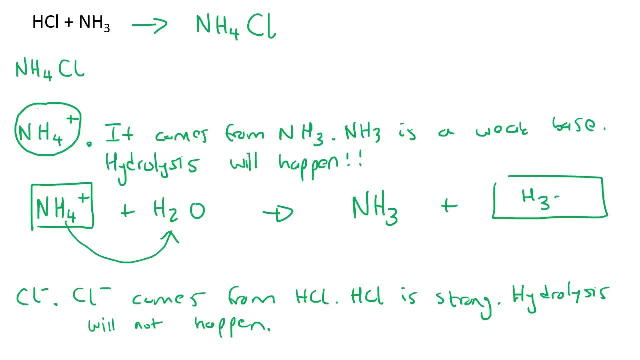 The water, of course, And so that will become H3O+. That is hydrolysis. Now it gets more interesting. We know that H3O+ is something that acids produce. That's something that acids produce, So it makes the pH go down. 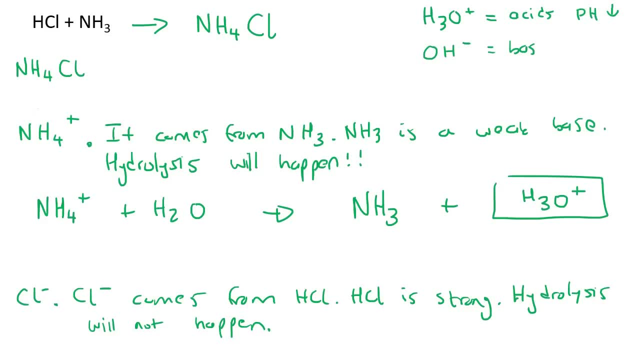 And we know that if you produce OH-, that is something that bases do And that makes pH go up. So what are we doing in this process? We are producing H3O+, So we are going to make the pH go down. So we can say that if you do a titration, 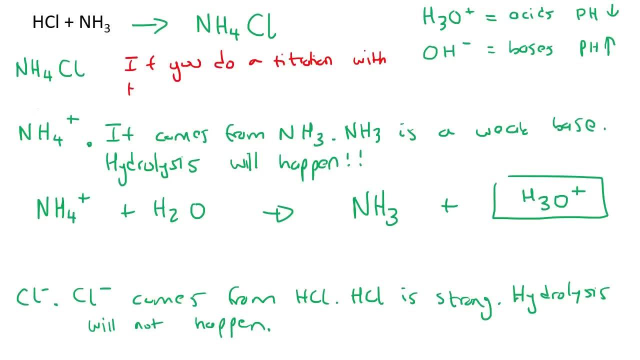 with HCl and NH3, the pH should be less than 7.. Will be smaller than 7. Because in the hydrolysis reaction that takes place, we are going to produce more H3O+ and that makes the pH go down. 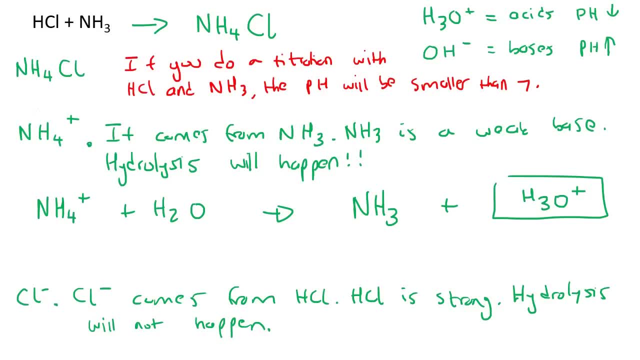 Because that's something that acids do. Now check this out, guys. I want to show you something else. Can you see that we have a weak acid? I mean a strong acid, my bad, a strong acid plus a weak base. 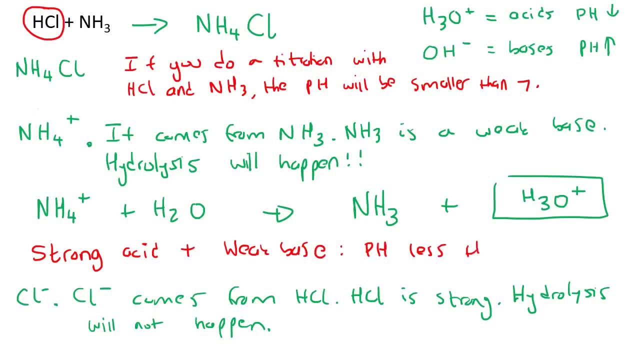 then the pH will be less than 7. Which is like saying more acidic. Now, I don't know about you, but that makes perfect sense. If you take a strong acid and you react it with a weak base, the acid is going to be the more dominant character. 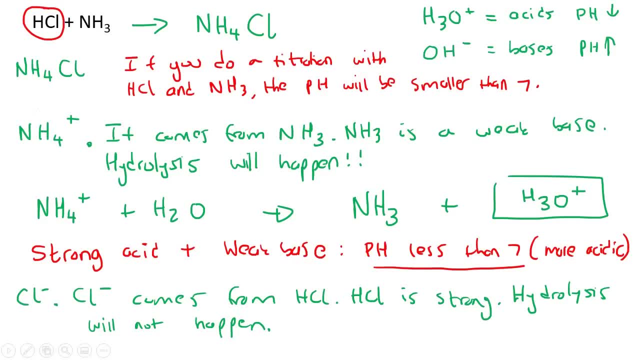 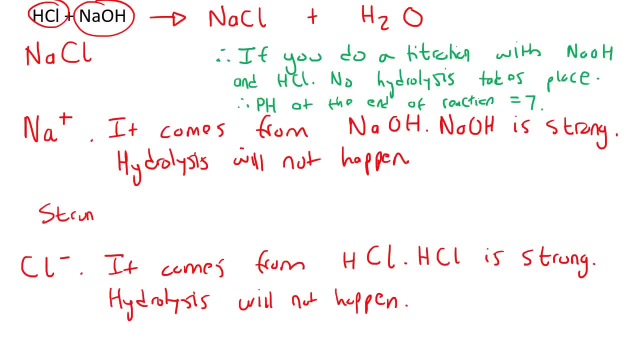 and so we are going to get a pH less than 7 at the end. That makes sense In the previous example, if you take a strong acid and a strong base, so a strong acid plus a strong base, then it makes sense. 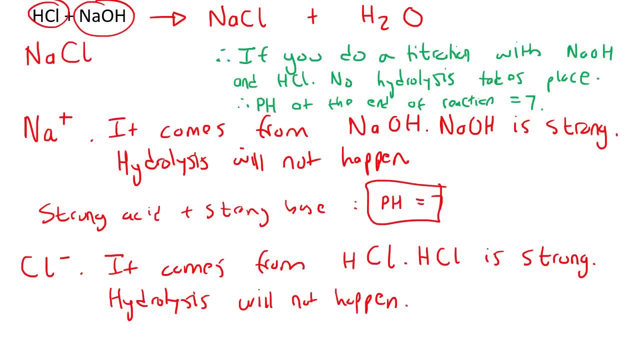 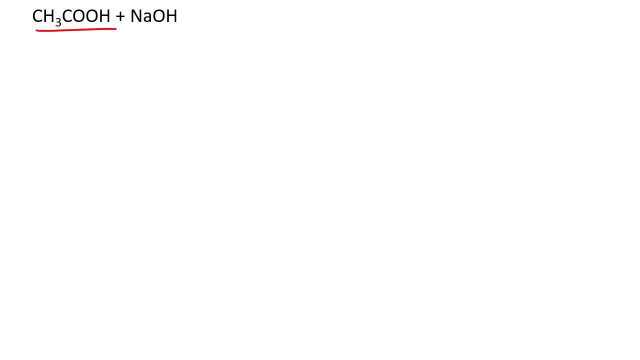 that the pH will be equal to 7, because they balance out. This is all during a titration, of course. Now let's do another example. So now we have an acid plus a metal hydroxide, so we know that that always gives us a salt. 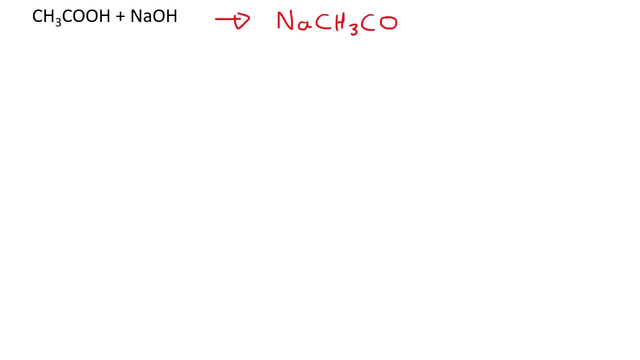 So now we have an acid plus a metal hydroxide. so we know that that always gives us a salt. So now we have an acid plus water, Then for hydrolysis or to be able to identify hydrolysis. 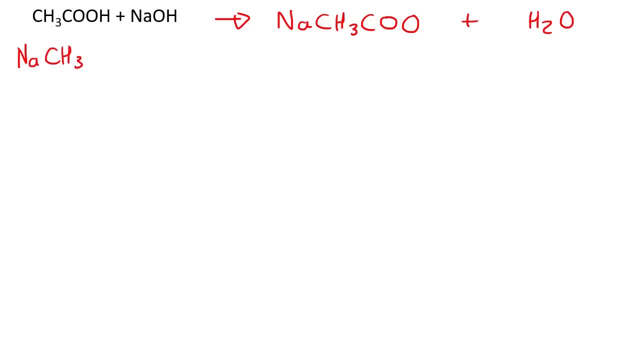 you look at the salt, which is the N-A-C-H-3-C-O-O, which is the N-A-C-H-3-C-O-O, and you break that up into its building blocks. Then you look and see: where did it come from? 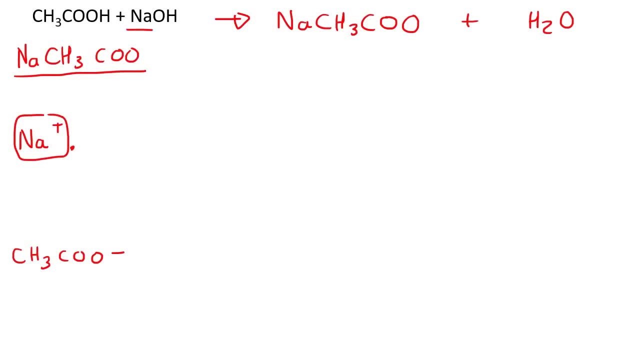 Then you look and see where did it come from. So if you look at this N-A-plus, it obviously came from N-A-O-H. So I'm going to say here comes from N-A-O-H, comes from N-A-O-H. 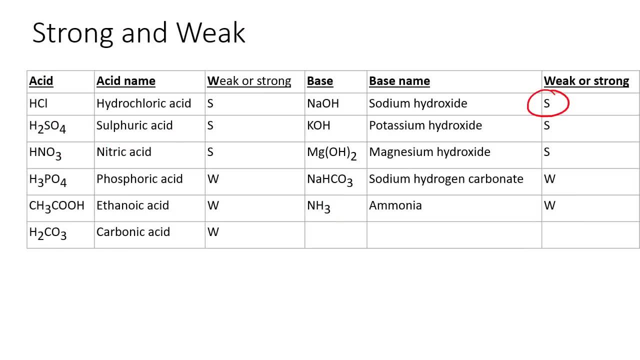 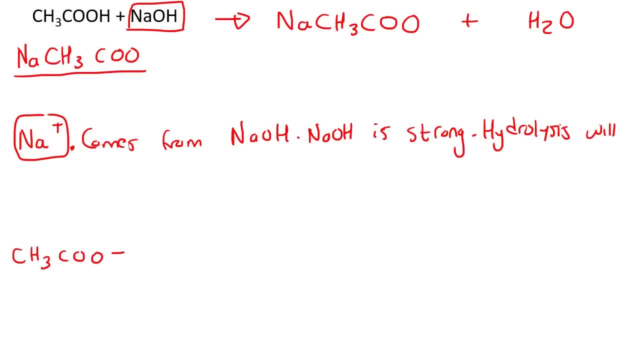 comes from N-A-O-H- We already saw is strong, and so therefore, hydrolysis, and so therefore, hydrolysis will not happen over there. Now let's have a look at the CH3COO-. Now let's have a look at the CH3COO-. 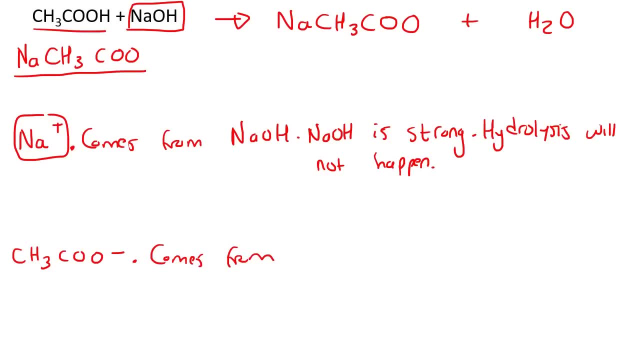 that comes from this one over here. CH3, or it's ethanoic acid- CH3COO- comes from CH3COO- Now, if you look at that, that is ethanoic acid, which is weak. It's a weak acid. 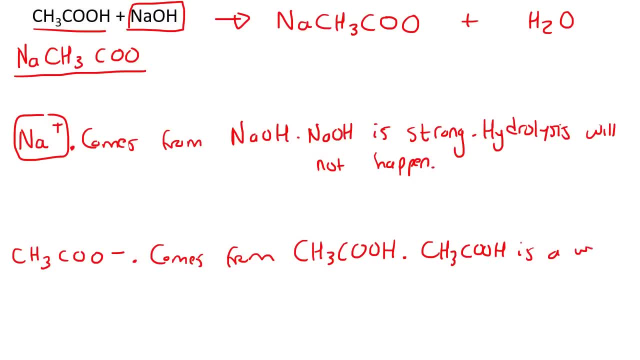 CH3COO- is a weak acid. So what does that mean? Hydrolysis will take place. It will happen. How does it take place? Well, what it means is that it means that this CH3COO- over there is not feeling. 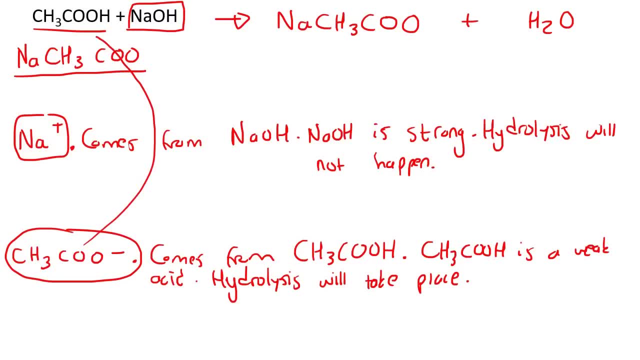 very comfortable. It's going to try and go back and become CH3COO-H. How does it do that? It reacts with water. So the hydrolysis reaction will look like this: It will react with water And we know that it's going to become. 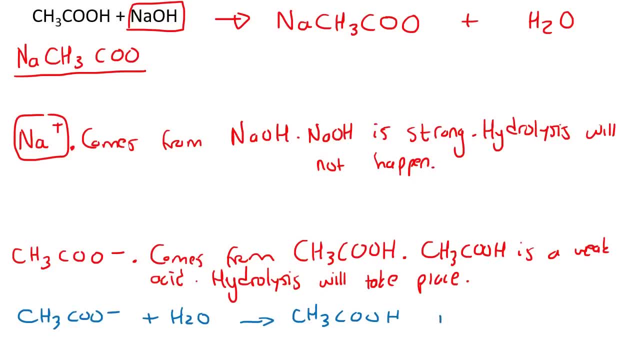 CH3COO-H. Now you've got to look carefully. Did the water molecule give a hydrogen Or did the water molecule accept a hydrogen? Well, well done. if you can see that it gave a hydrogen, So that means the water molecule. 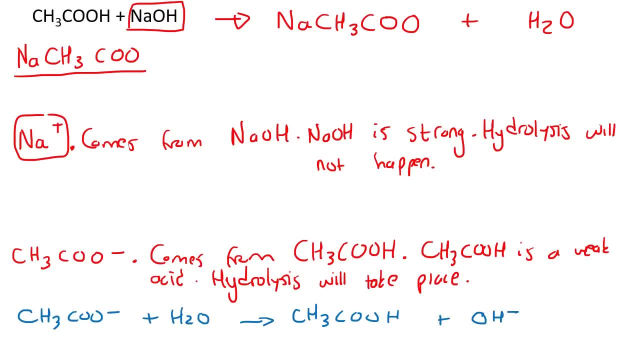 is now OH-. So look at this, guys: We are producing OH-. Now that is something that bases do, And so the pH is going to go up. We can say that the OH- concentration is increasing, And so, therefore, that's something that bases do. 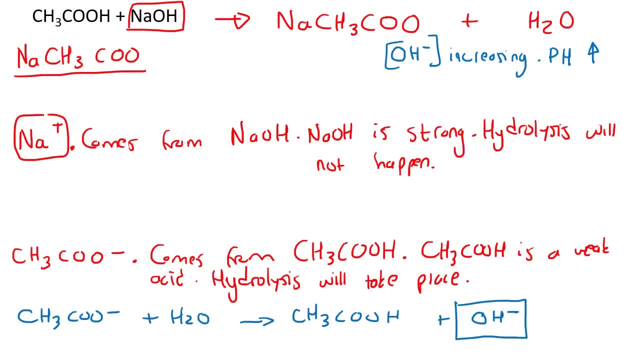 And so the pH is actually going to go up. So, therefore, if you do a titration with CH3COO-H and NaOH, then the pH will be larger than 7. And it makes perfect sense. We've got a weak acid. 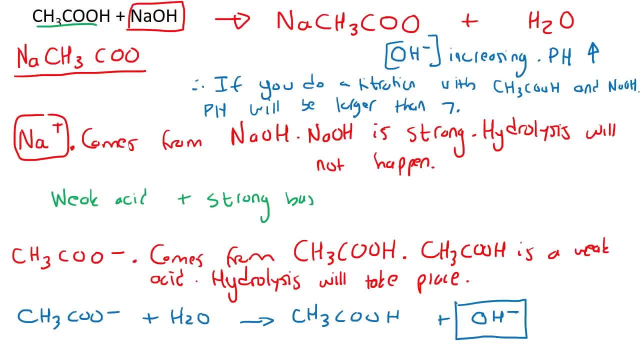 plus a strong base, Then that means that the pH will be larger than 7. And that's something that bases do, So it makes sense. If you've got a weak acid and a strong base, the strong base will dominate, And so your pH at the end will be larger. 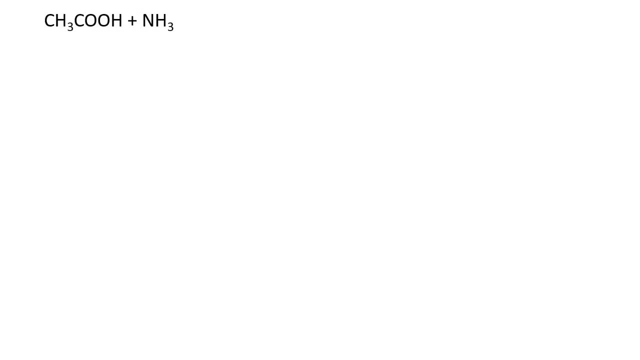 than 7.. And then, lastly, we are going to react these two together. So we know that if you take an acid and an ammonia, you make an ammonium salt Or ammonium salt- yeah, I said that twice- NH4CH3COO. 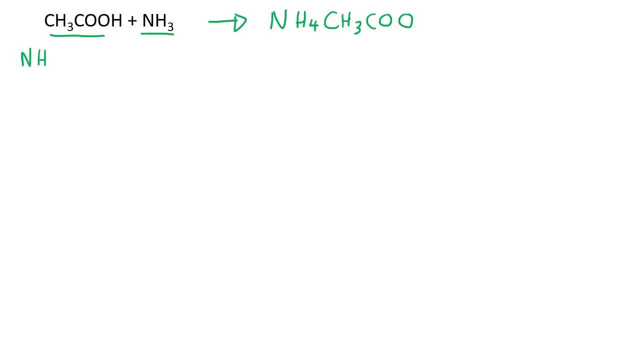 So what you do for hydrolysis is: you take that salt, you break it up into its building blocks, which is NH4 positive and CH3COO- Then you see where they came from. So we know that this one NH4+ comes. 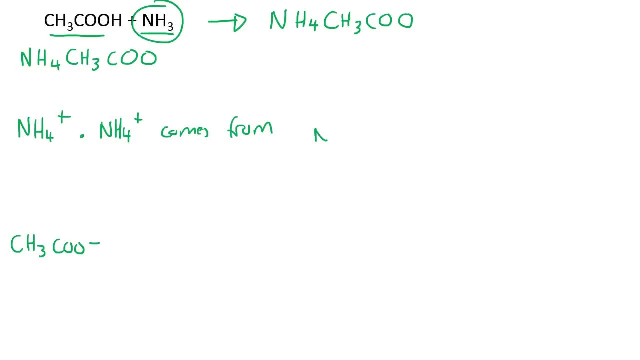 from. it obviously comes from NH3. Now, NH3 is weak, So hydrolysis will take place. Great, Let's look at the next one. So we know that this one comes from the ethanoic acid, which is this part over here. 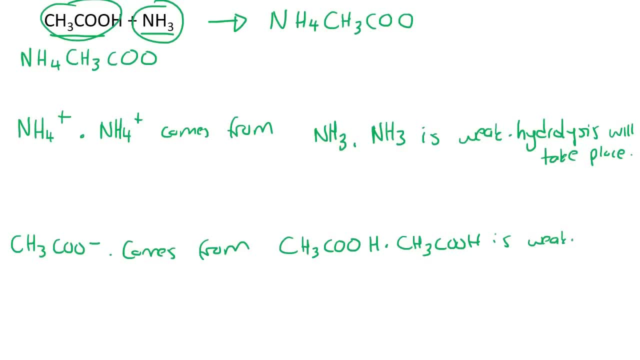 We know that that is weak, So hydrolysis will take place for this one as well. So we're going to have two sets of hydrolysis reactions taking place. So we know that this thing is going to react with water And it's going to try to go back to what it was. 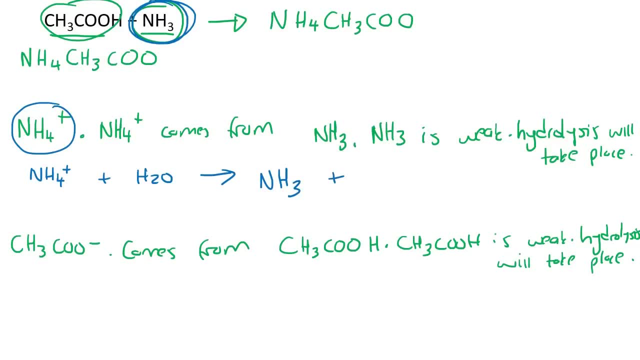 in the beginning, which is NH3.. So can you see that a hydrogen is going to be given to the H2O molecule, So the H2O molecule should become H3O+. Now can you see we are producing H3O+. 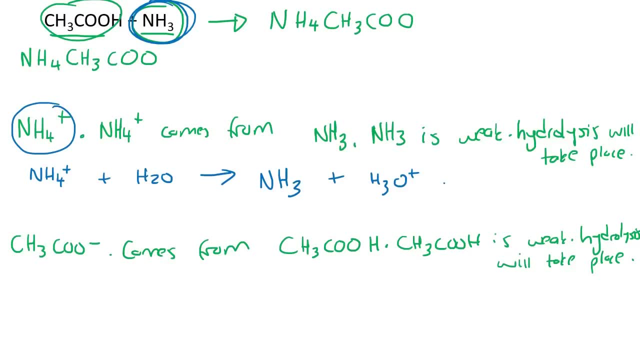 which makes the pH go down because that's more acidic. So therefore, pH will drop Because we are making more H3O+. Now let's look at this one over here. So now what we have is this one is going to react with. 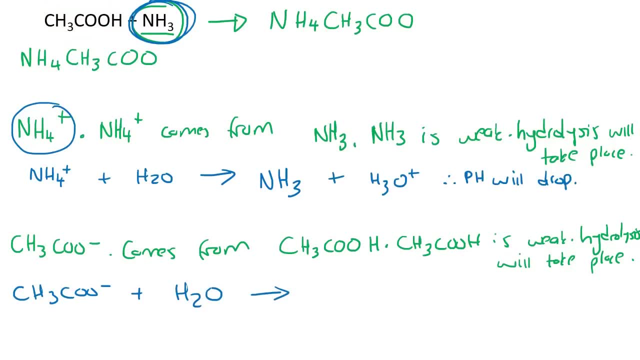 water. It's always water, hey, And that's going to try to go back to what it was originally, which is this one over here, And now you've got to look carefully. Can you see that this water molecule gave the hydrogen away? 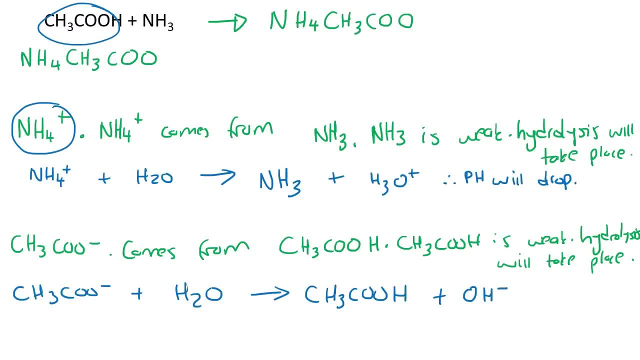 So the water molecule will now become an OH- And we know that that is something that bases do, And so that is going to make the pH- it's actually going to make the pH- go up. Therefore, pH will rise. So we've got a. 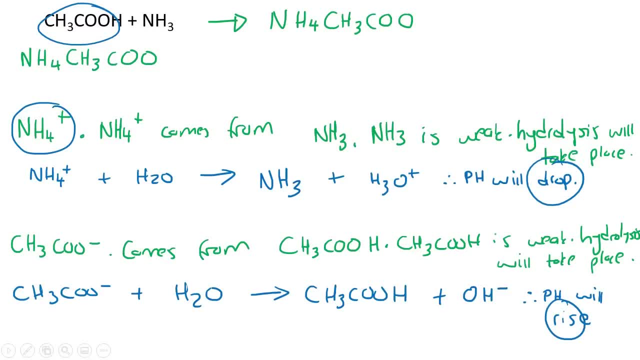 pH dropping and we've got a pH rising. So what does that mean? If you look at the overall effect, the pH will remain at 7.. Therefore, pH will be equal to 7.. So this makes sense, because if you take a weak acid, 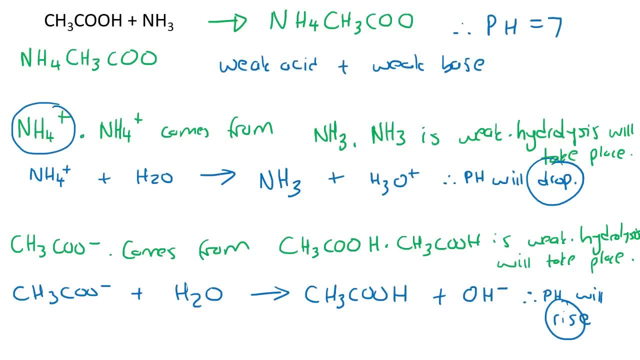 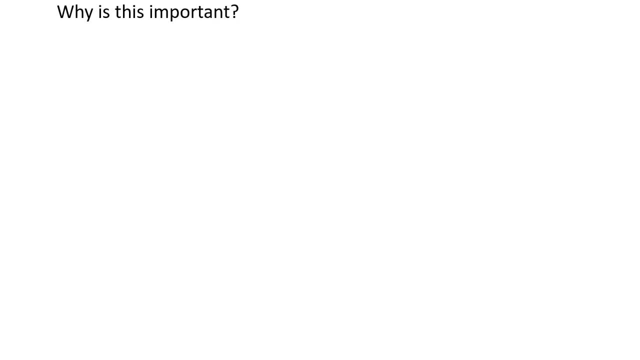 plus a weak base, then they're just going to cancel each other out, And so the overall pH will just be equal to 7.. Now why is this important? It is important because of the following: If you do a titration in real life, so let's say if you do. 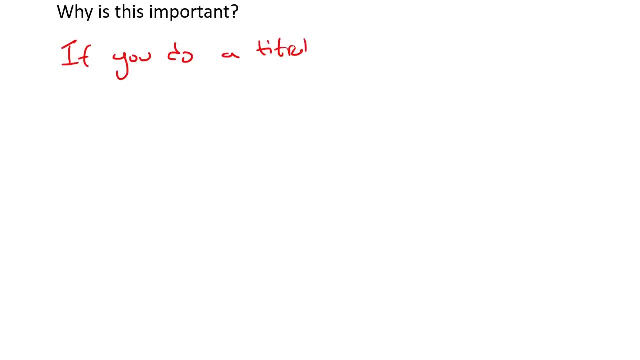 a titration with a strong acid plus a strong base, what would the pH be at the neutralization point? Well, we know that the pH would be somewhere around 7.. But now, when you do a titration in real life, how do you know when it is complete? 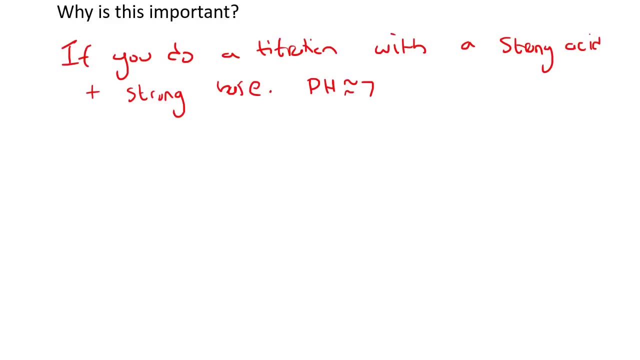 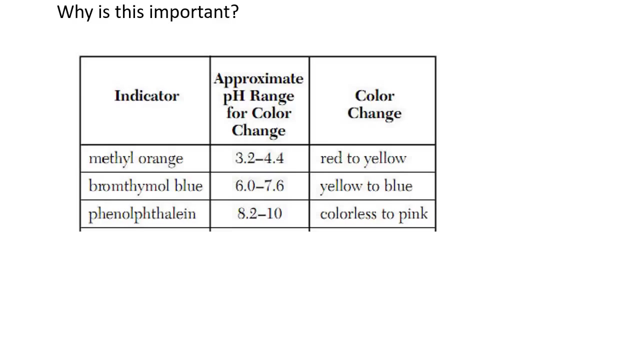 It is complete when the color changes or the indicator changes color right. So you need to make sure that you are using the correct pH indicator, Because you get three different or three main types. there are others, but we know that there is an indicator called. 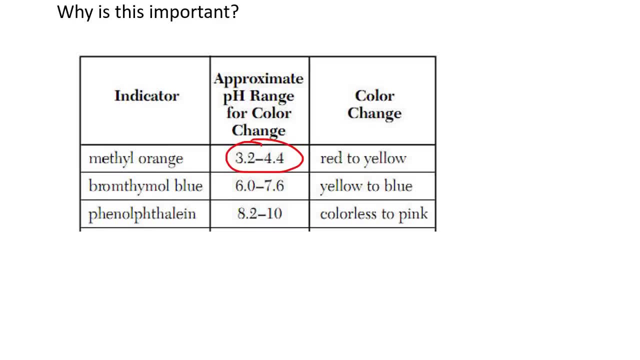 methyl orange, which changes pH at about there. Then you get bromothymol blue, which changes pH over there, and then you get that word, eh, Phenolphthalein, whatever it is, which changes pH over there. So if you take a strong acid, 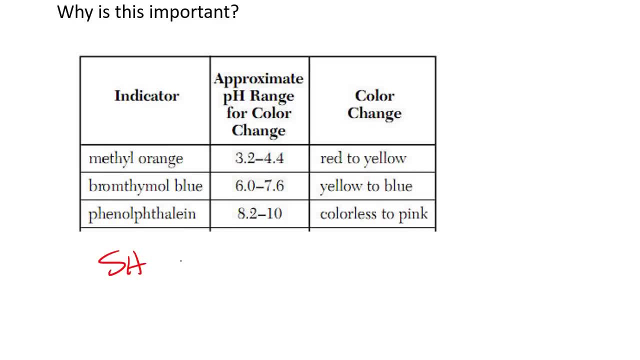 I'm just going to say SA for strong acid plus a strong base. then we know that the pH changes at about 7.. So it would make sense that you use bromothymol blue for that type of. so use bromothymol. 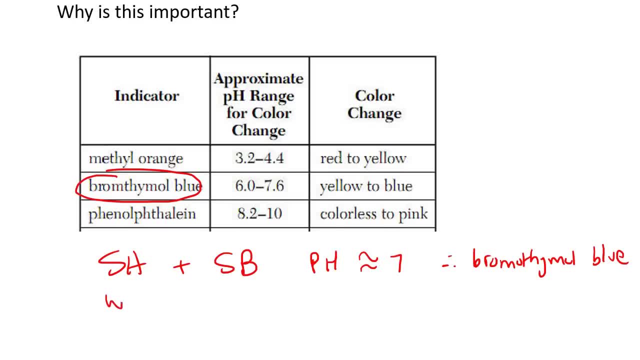 blue. If you take a weak acid plus a strong base, then the base is going to dominate. Now, bases have a high pH, so your pH will be somewhere around 9,, I guess. So then you would use phenol. oh my goodness. 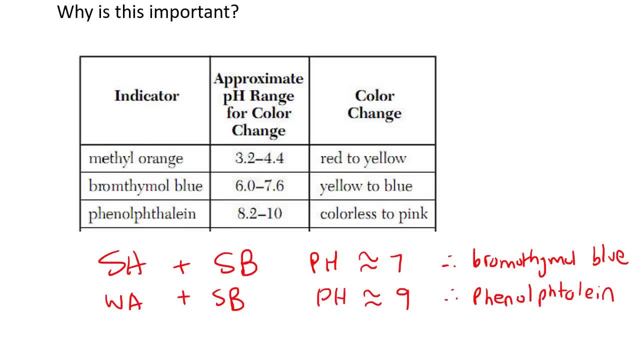 phenolphthalein. And then, of course, if you take something like a strong acid and a weak base, then the acid is going to dominate, So your pH would change at around I don't know 4.. So then you would use methyl orange.